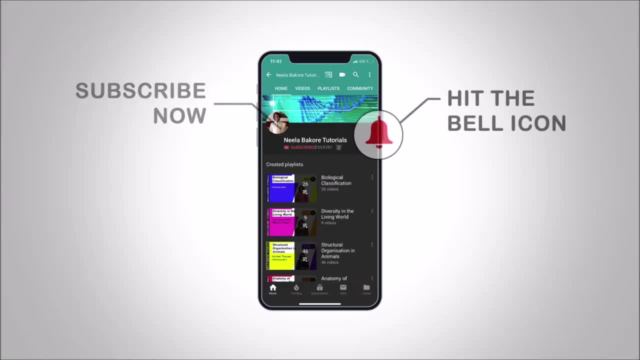 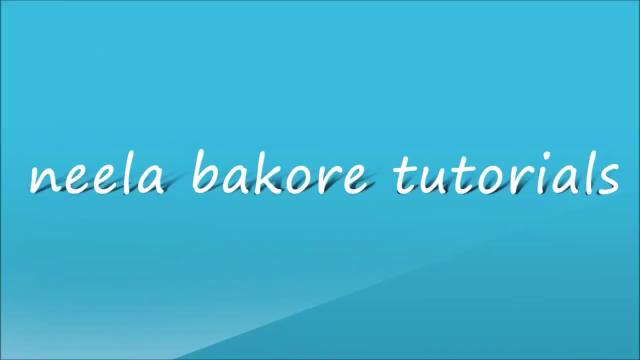 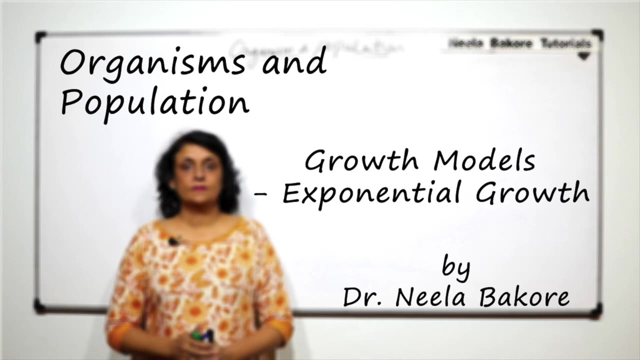 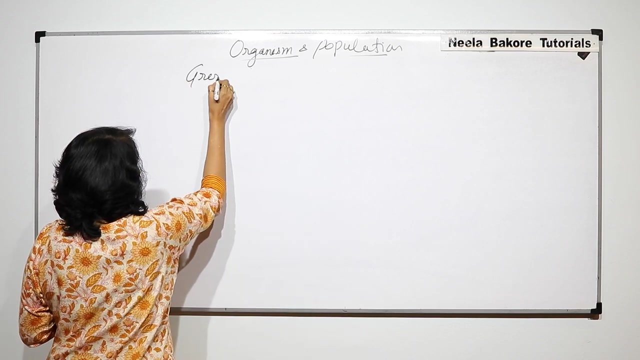 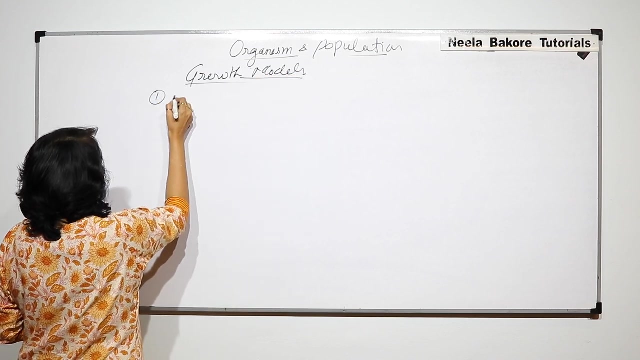 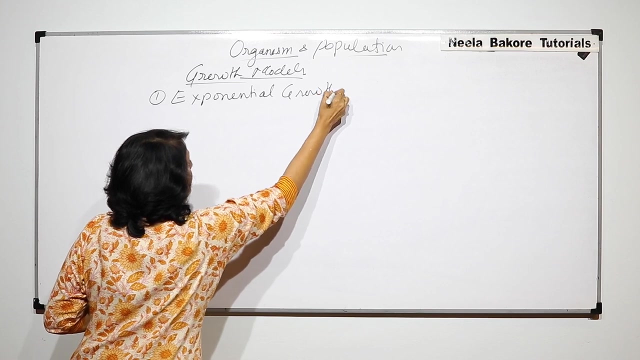 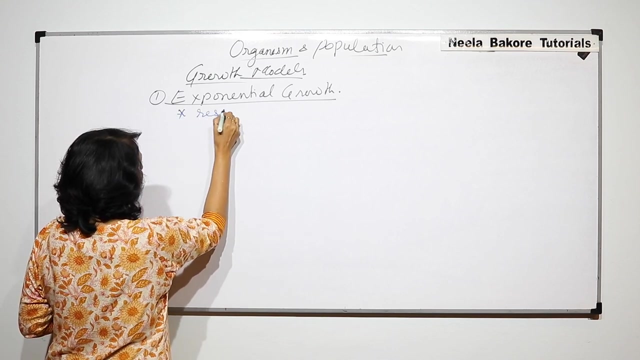 Hit that subscribe button and bell icon so you never miss an update from neelabhagore tutorials. In this video we'll talk about the growth models, And the first one that we are talking of is known as the exponential growth. Now, this type of growth is seen when the resources are unlimited. 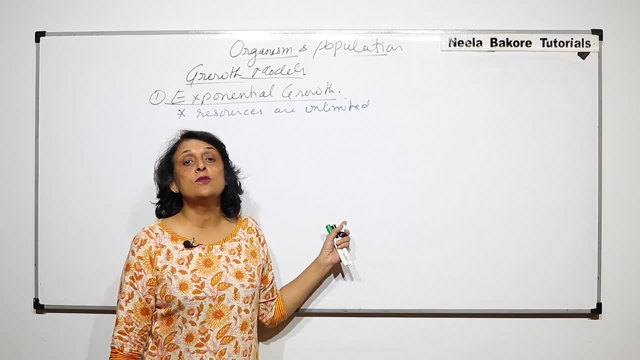 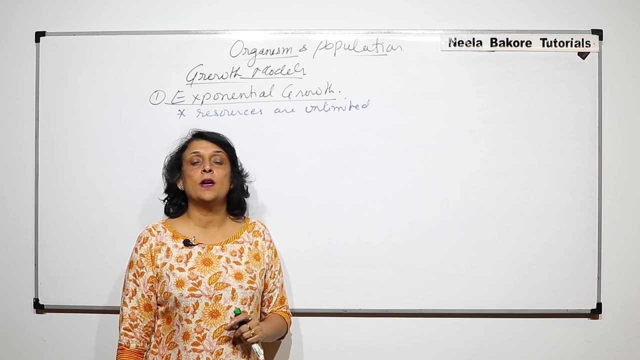 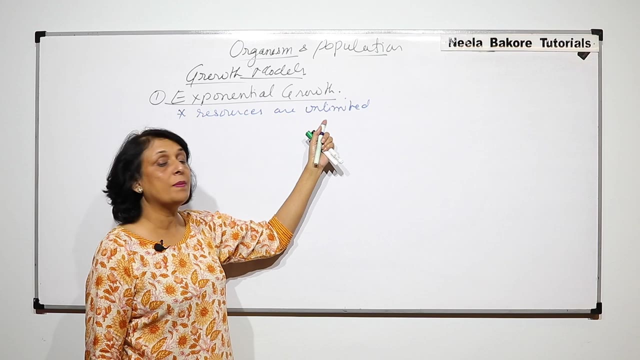 And we have already discussed this point- that this is not a naturally occurring process In nature, something, some resource is definitely going to become a limiting factor and that limiting factor will regulate the growth. But in this case we are talking about a situation where the resources are unlimited. 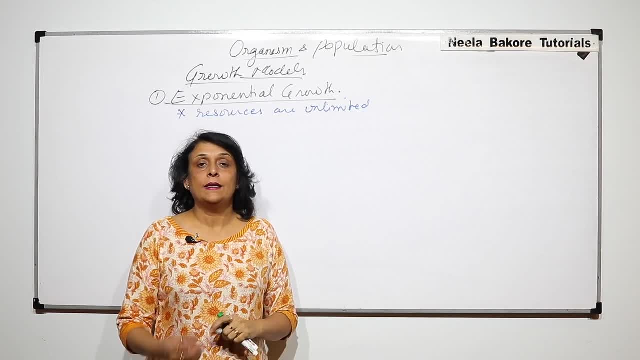 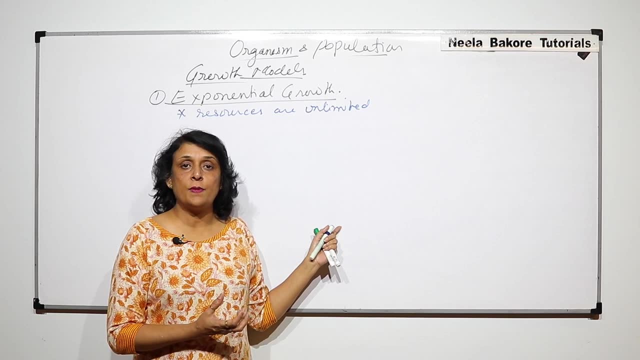 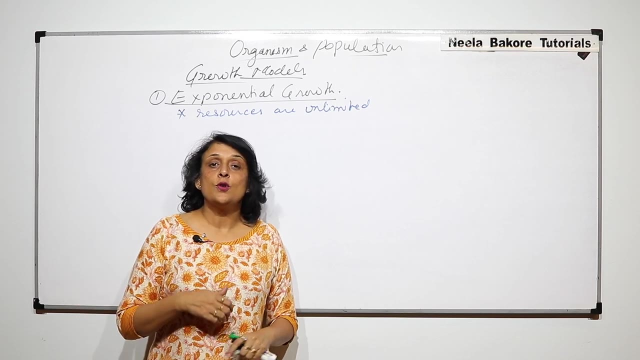 This type of condition is seen in case of labs. That means if you are growing a bacteria in a laboratory condition, say in a petri dish, then because we are supplying the nourishment, we can move those bacteria from a small amount of petri dish to a bigger one or into a bigger jar. also. 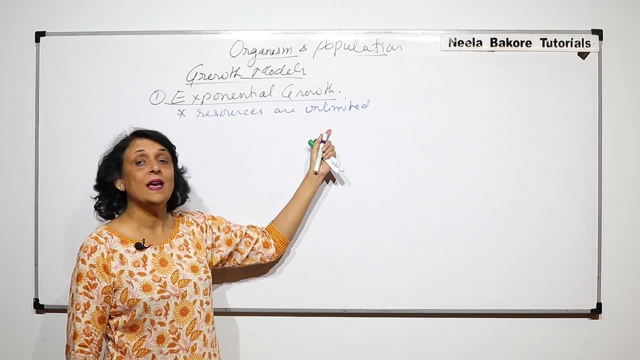 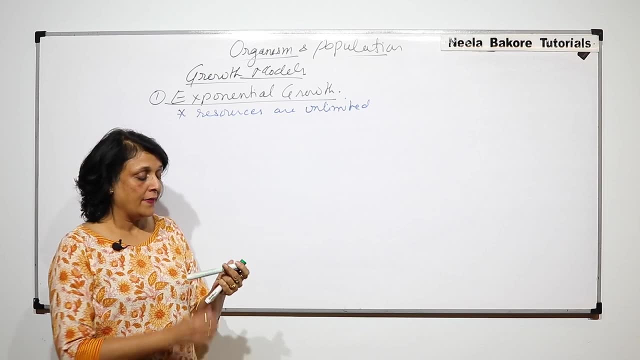 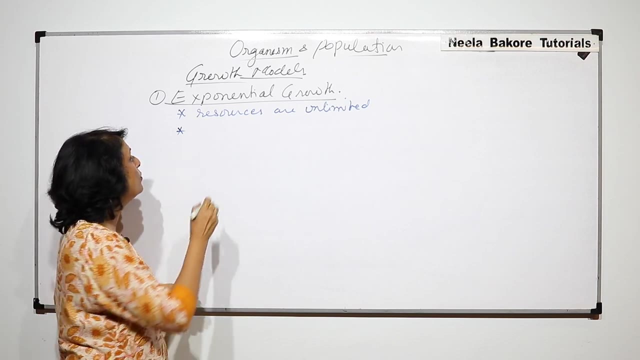 So the space, nutrition, everything is going to be unlimited for those bacteria. Then in that case, the growth which is seen is known as the exponential growth. The second thing is, in this growth, one more factor which is taken into account is that 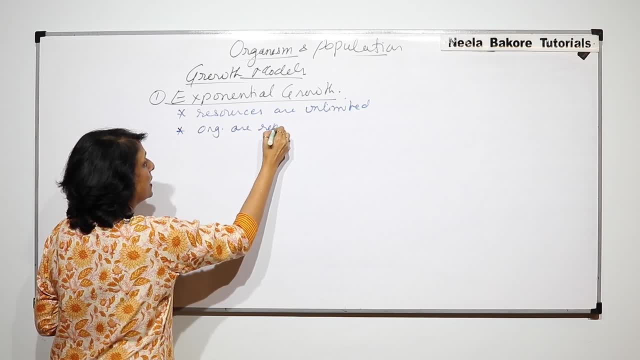 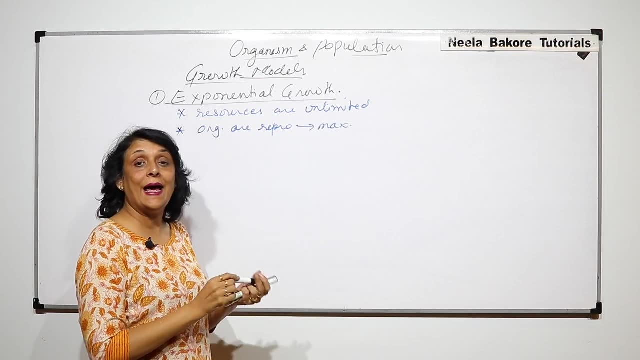 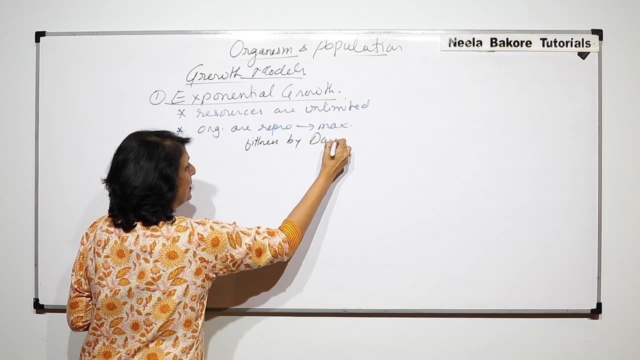 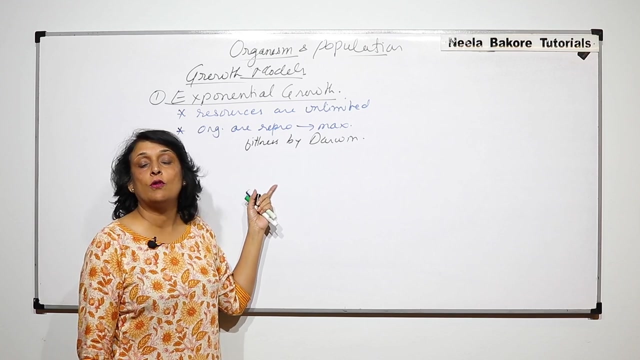 the organisms are reproducing to their maximum capacity. Okay, And this is what is known as the fitness by Darwin. Darwin said survival of the fittest, So the fitness or the fit word is used for the organisms which are able to utilize their reproductive potential to the maximum. 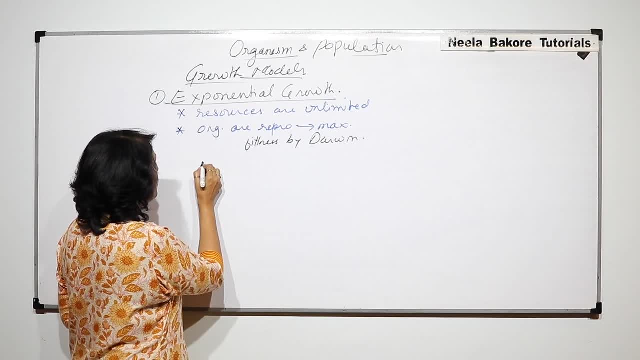 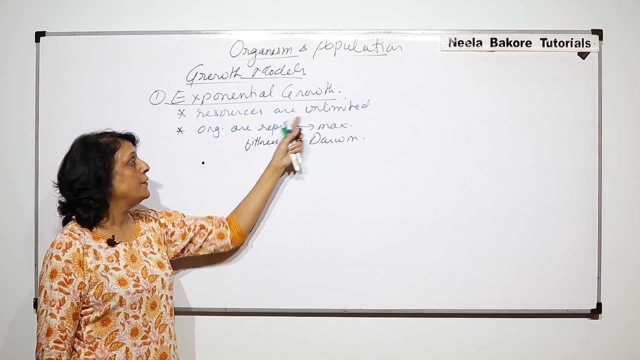 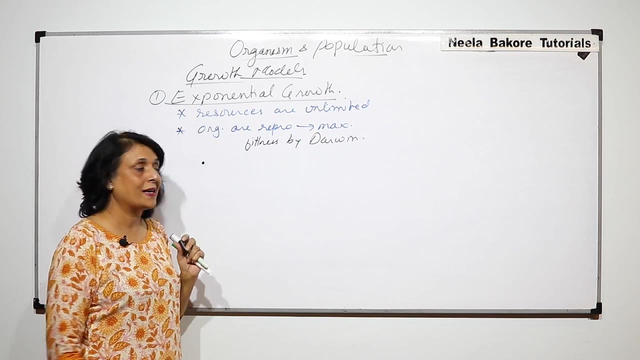 So these are the conditions. Now, if we want to find out The growth increase or decrease, like, how much is the growth if resources are unlimited and the fitness, or that is, the reproductive potential, is utilized to the maximum? The population size is represented by n. 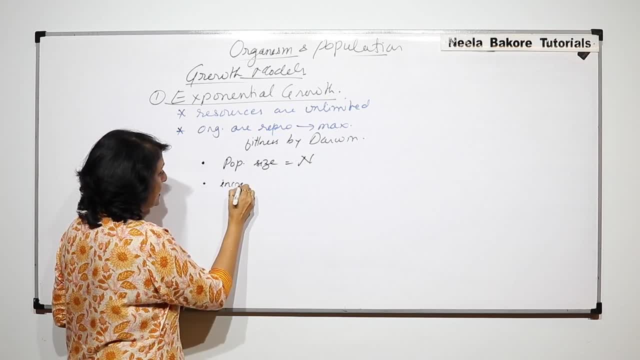 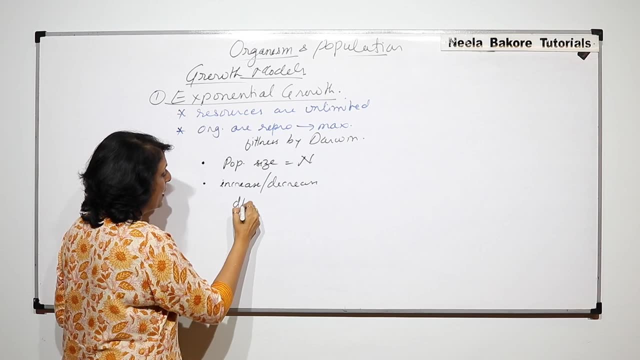 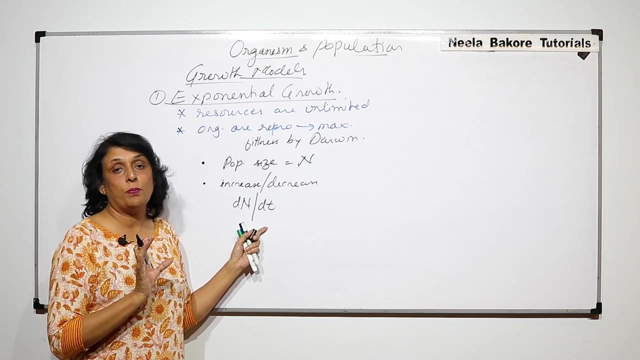 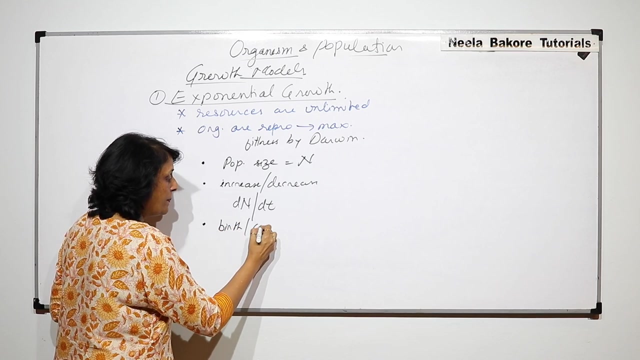 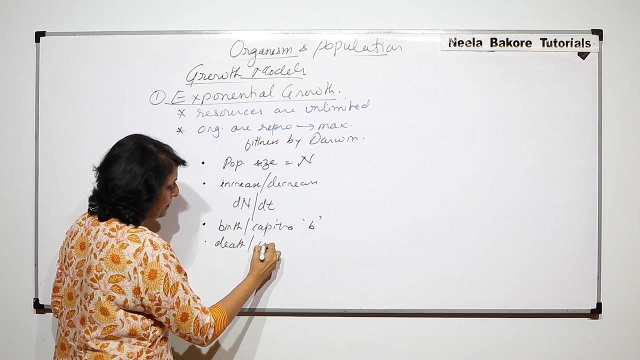 And if we want to find out the increase or decrease in this population size, it can be found out by dn upon dt. t is the time period in which we want to study the population increase or decrease. Here the birth per capita is taken as small. b and death per capita is written as small. 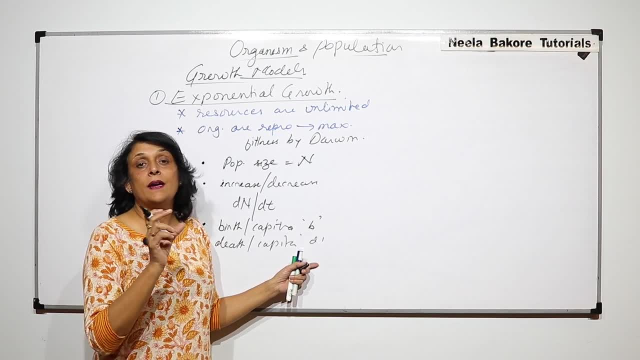 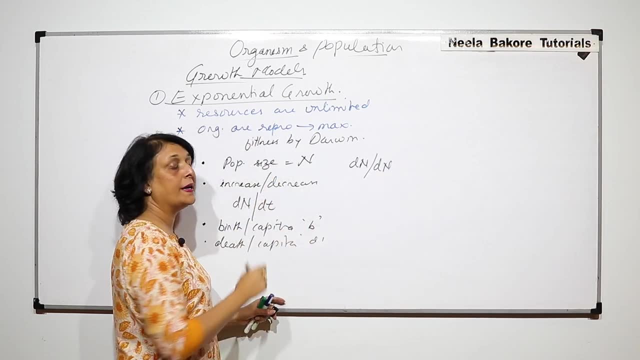 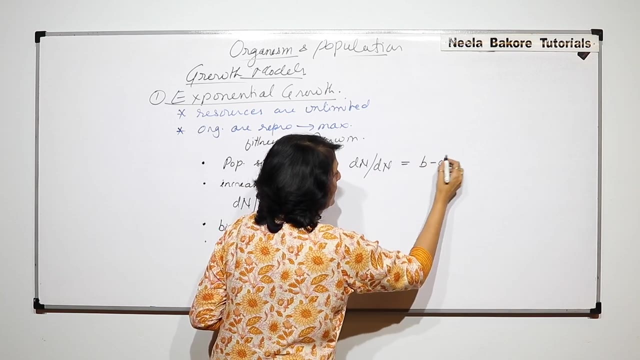 d. So if we have to find out, or if we make an equation, Then It is going to be dn upon dt. That is, we want to find out the increase or the decrease, Then it is going to be birth per capita minus death per capita and the actual population. 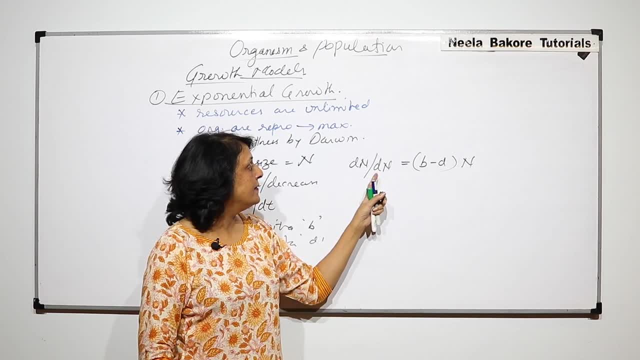 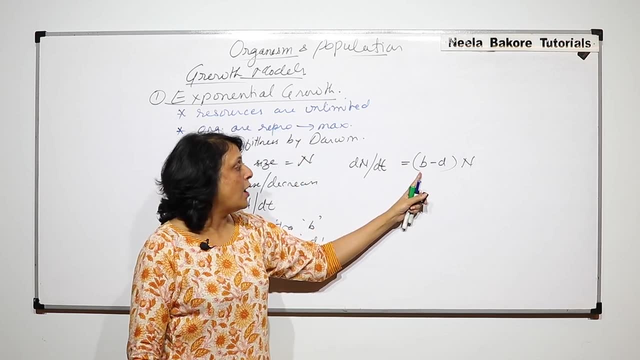 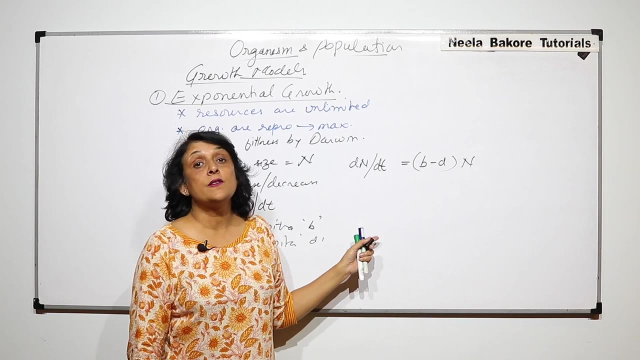 So this is the original population which is existing in this time period. So it is dn upon dt. So in the given time period, How many added per capita And how many died, How many per capita? So that and the existing population. 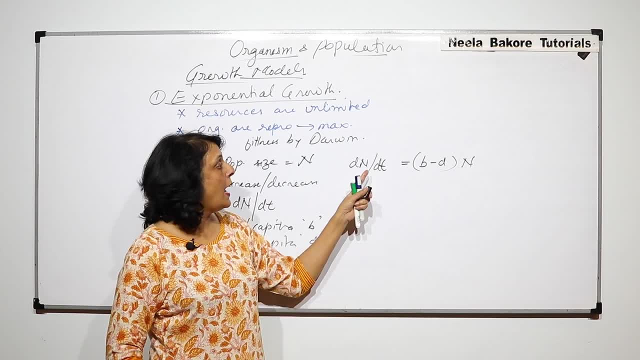 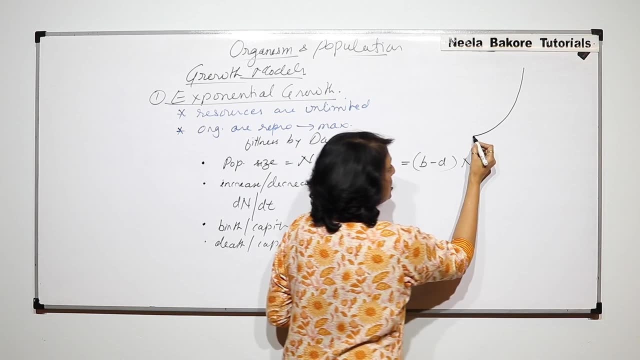 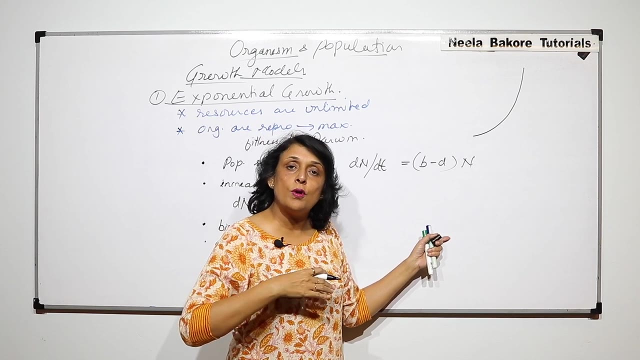 This is going to give us the exponential growth. And if we plot this type of growth, we will get a curve in which initial growth is going to be small or slow And then, because resources are unlimited, it's going to grow in an exponential manner. 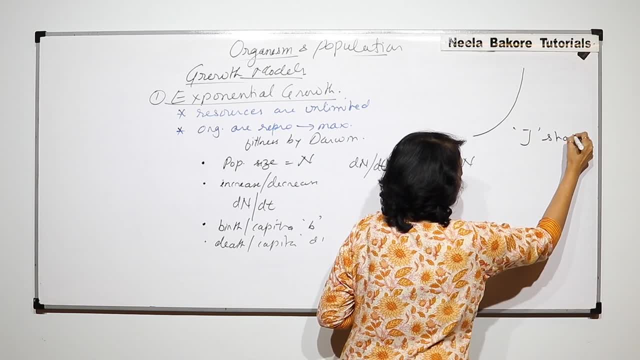 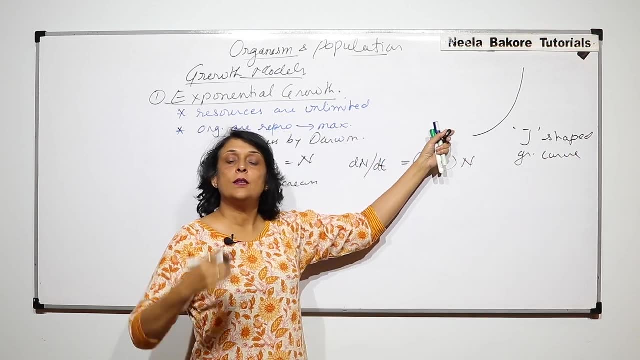 And this is known as J shaped growth curve. So this is the growth curve And this is the growth curve And this is the growth curve. So this is the growth curve And as the curve indicates that population is going to grow and grow, and grow continuously. 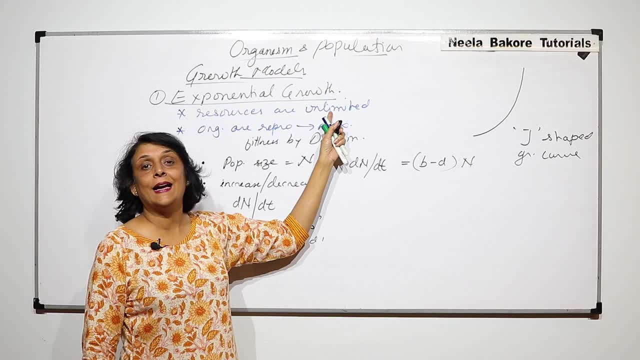 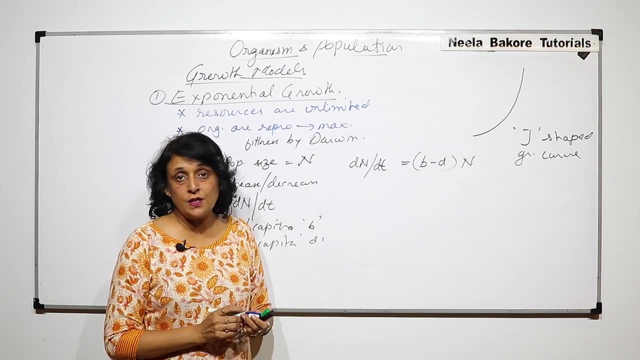 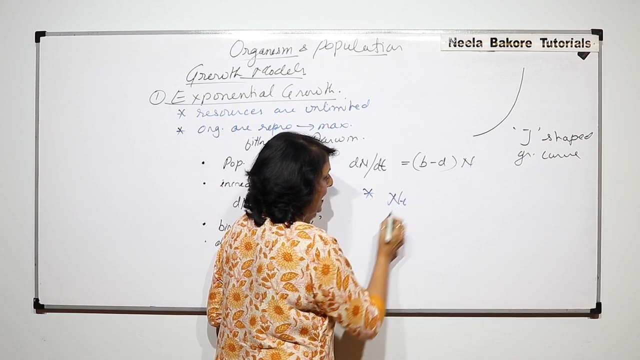 And this is possible only because of the factor that there's nothing which is limited. If we want to do a mathematical expression of this using calculus, then our equation is going to be slightly different. The equation is written as: nt, That is the growth after time period. 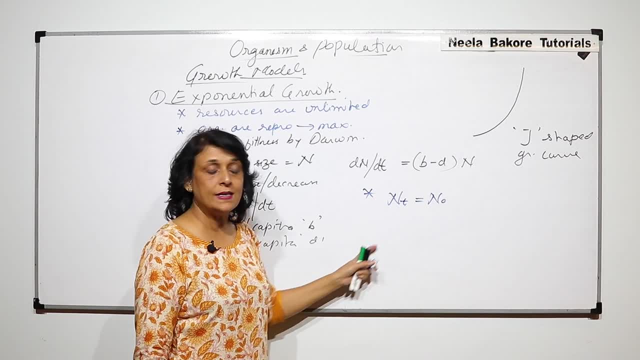 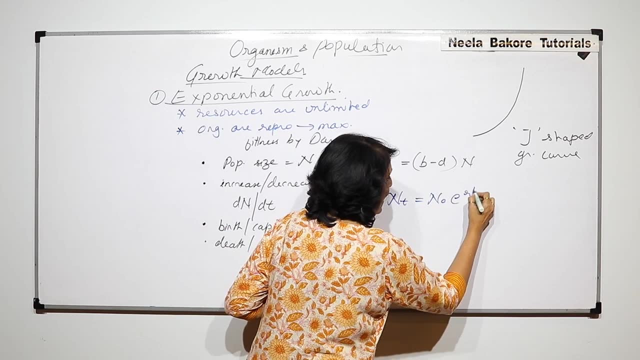 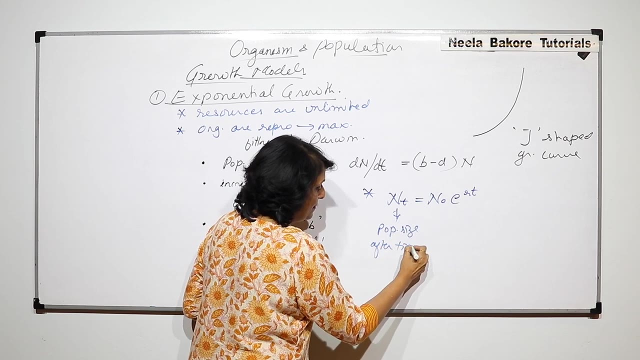 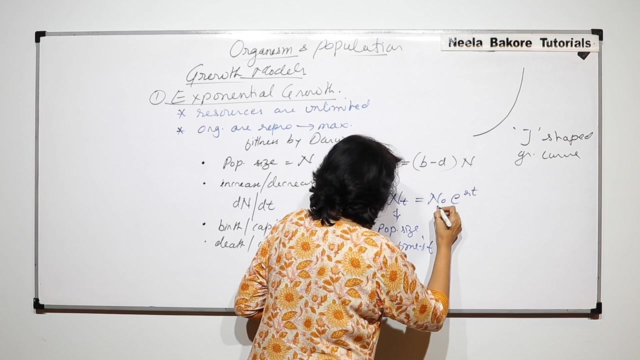 And t will be the original population size. That means the population size at that time period when we are starting that particular thing And Ert. So this is the population size after time t. After time t And n0 is the initial population. 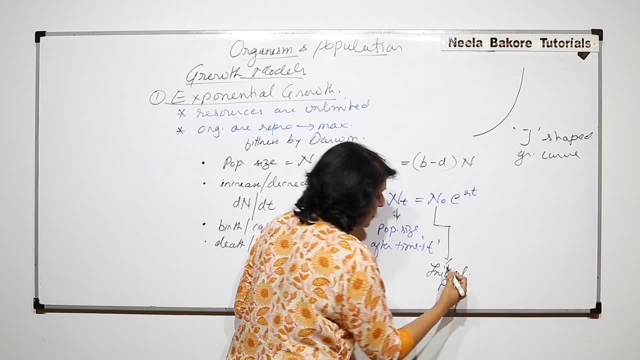 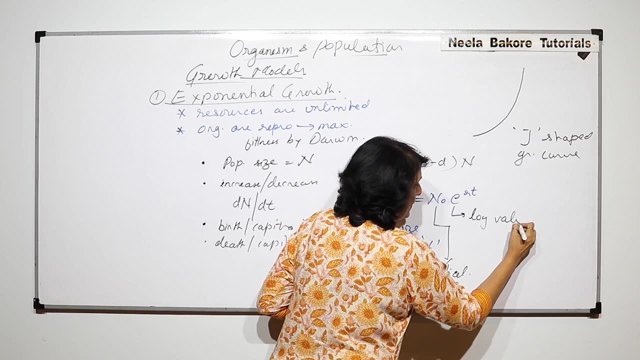 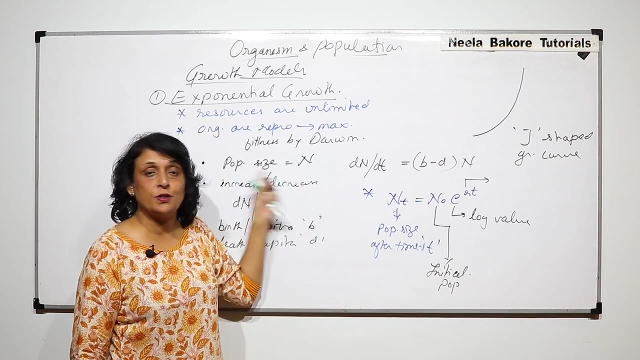 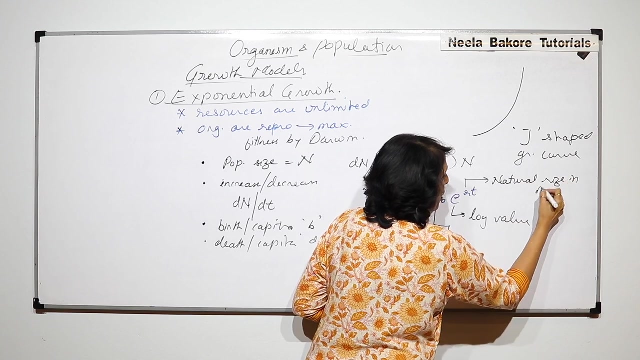 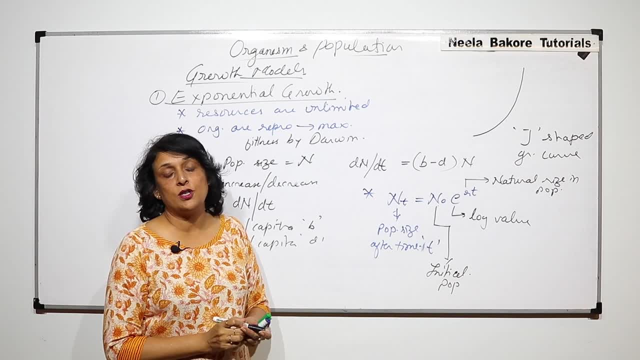 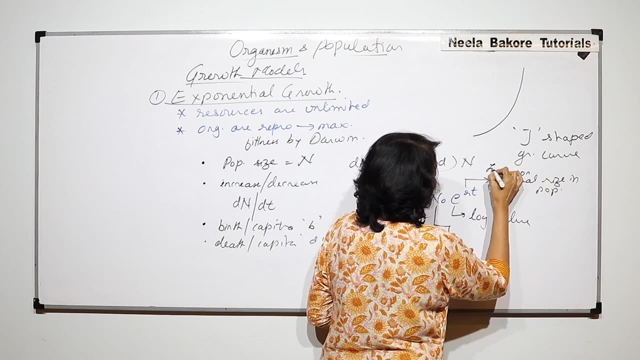 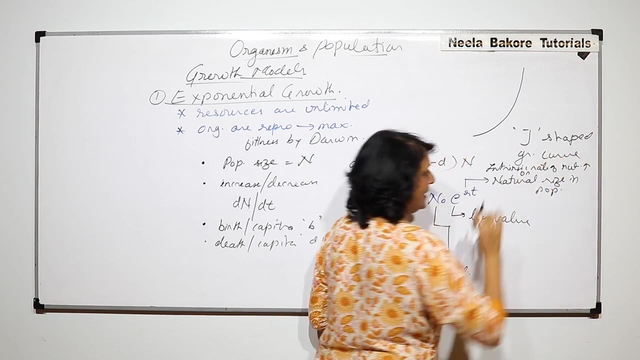 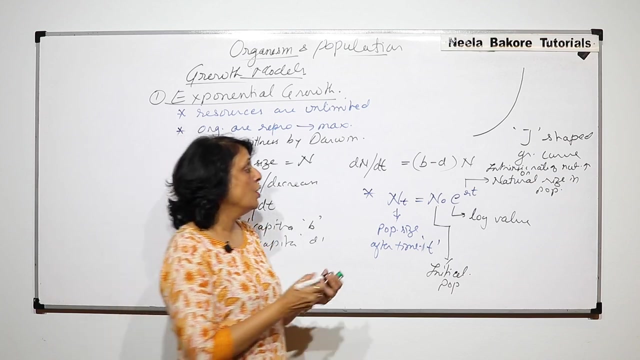 And this is because of the reproductive potential. It is also known as the intrinsic rate of natural growth of natural growth, so we can also write it as intrinsic rate of natural increase. this is basically the fitness. that means. what is the reproductive potential that the organism is able to use? and T is the time period in which we want to find out. 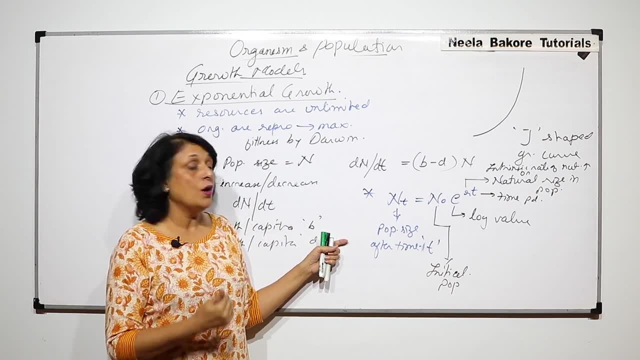 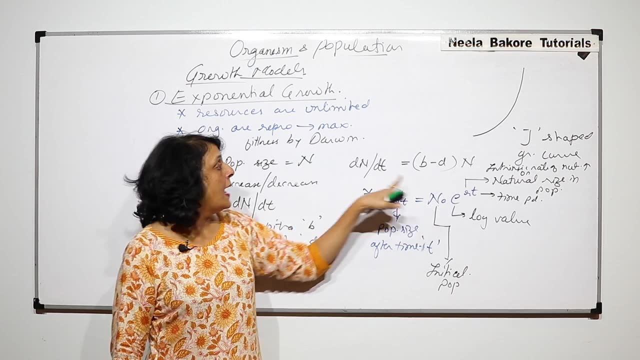 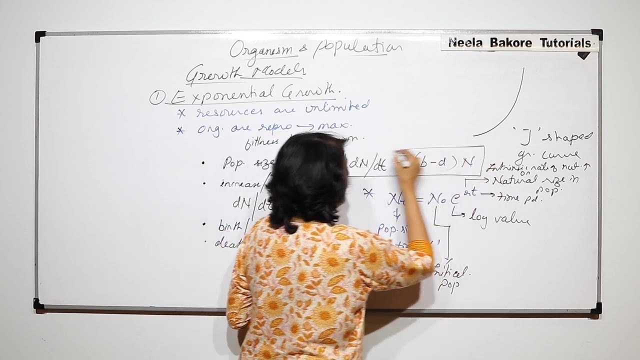 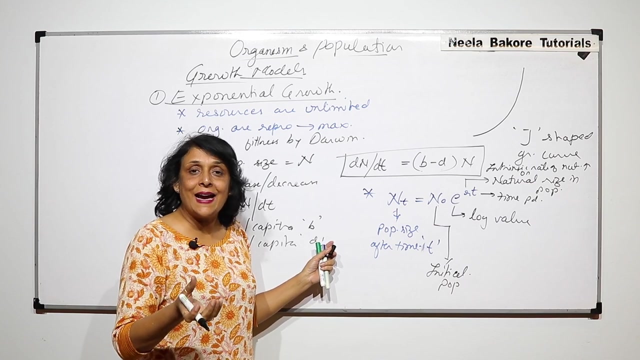 the change in the population size. so if we just use the mathematical expression, our equation is going to change, because here we are using the log value and in simple way it can be like this: or we can change this equation also: birth per capita minus death per capita, that means how many actually get added to the 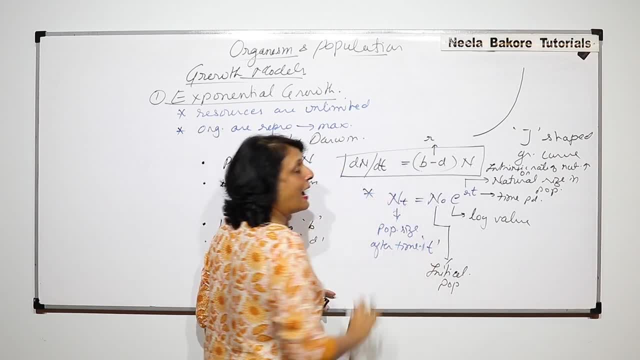 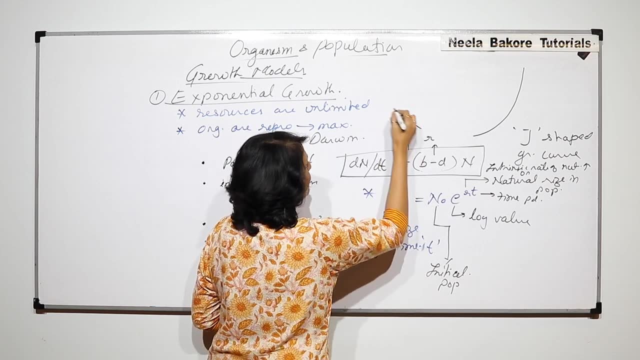 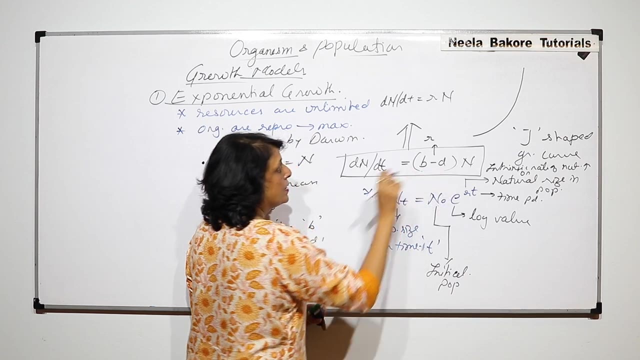 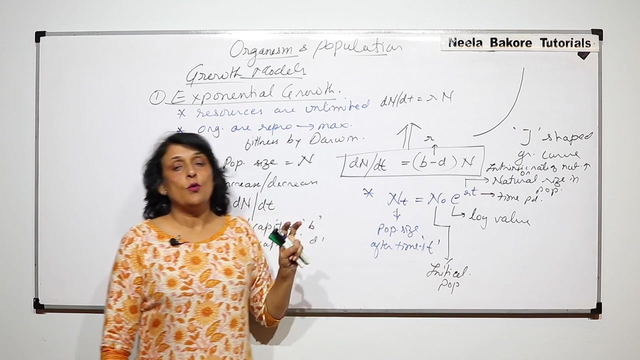 population. so this is nothing but the R, that is again the intrinsic growth. so our equation can change. this one can be written as DN upon DT and it will become RN, because B minus D is nothing but this R. that is the reproductive potential. so we can do it in a simple manner or using the